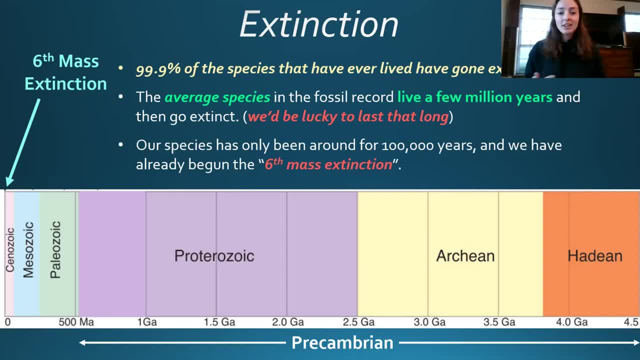 history and why extinction occurs and how it drives evolution and a lot of other things. just about extinction in general. But if you want to know a little bit more about what's happening currently- that's classified as the sixth mass extinction- you can go to the link in the description below. 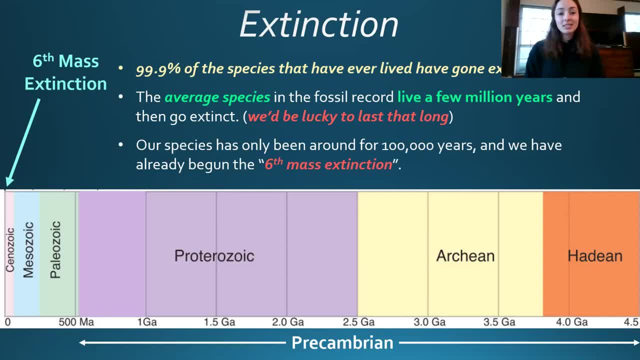 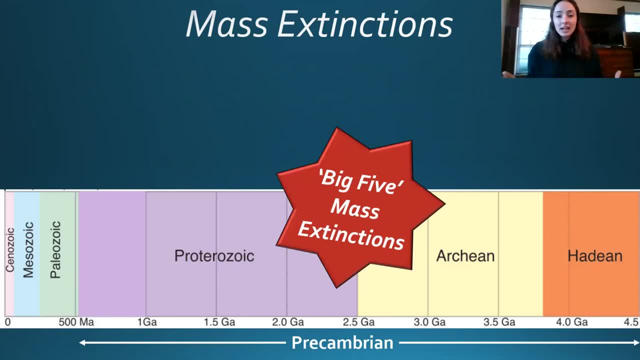 You can watch my climate video or I might make a video all about the sixth mass extinction in the future, But for this video let's get into the big five mass extinctions Now. this timeline of earth's history down here at the bottom shows from the beginning of earth's history at 4.5. 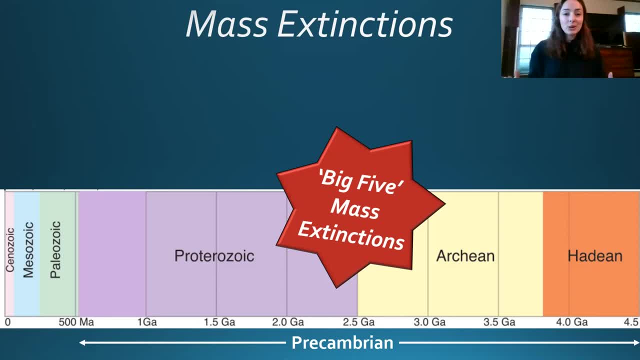 billion years ago, at the right of the screen, in the Hadean, to the Cenozoic, or now at zero million years ago. You might think that these big five mass extinctions would spread out periodically throughout this timeline. However, they are located in the Ordovician. 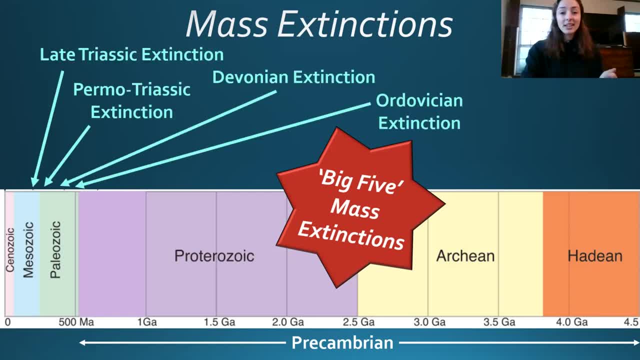 the Devonian, the Permatriassic boundary, the Late Triassic period and the Cretaceous-Tertiary boundary. These five mass extinctions are all clustered in the Phanerozoic, which includes the Paleozoic, Mesozoic and Cetozoic eras, And the reason is just because there wasn't a lot of. 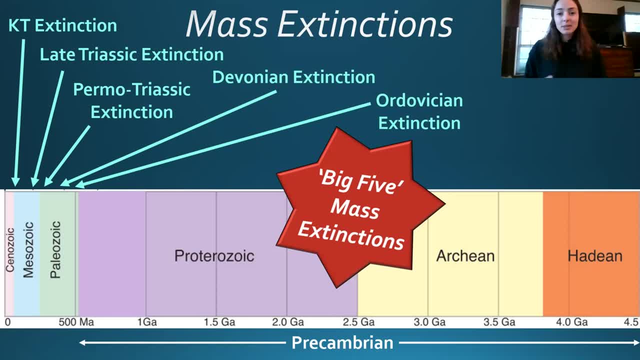 life. before that There was basically bacterial species, but they're hard to have really a fossil record to follow and to find extinctions in, And so the big five mass extinctions that we know of and have the most evidence for are located at these points. 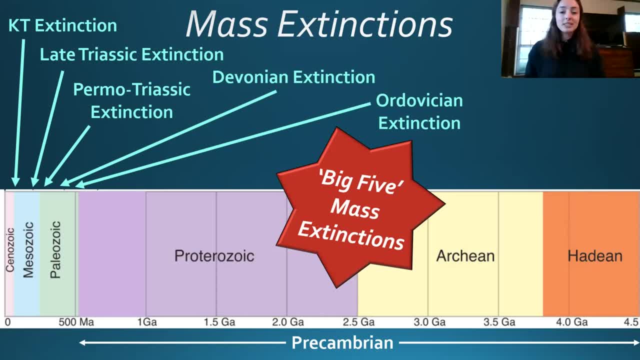 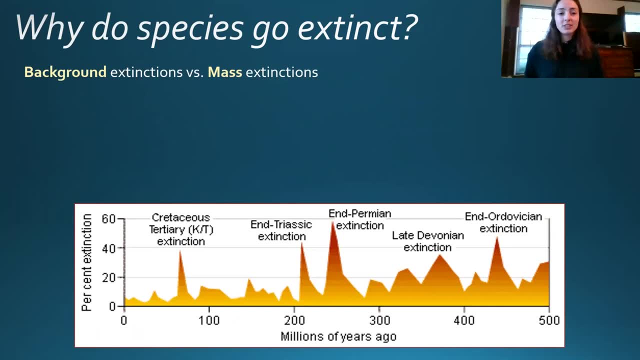 It's in the timeline And we'll be focusing on these in terms of mass extinctions. But before we get to that, we need to talk a little bit about why species go extinct. Mass extinctions aren't the only kinds of extinctions. There are also what's called background extinctions, As we see. 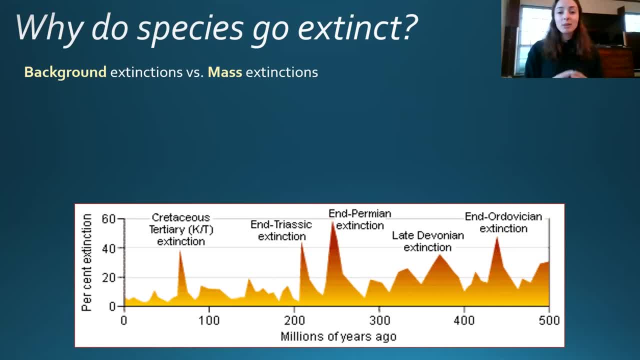 on the lower part of this slide we have extinction rate plotted against millions of years ago And this shows these five big peaks showing the mass extinctions we just listed. However, they're not the only extinctions going on. Extinction rate is still happening along the background. 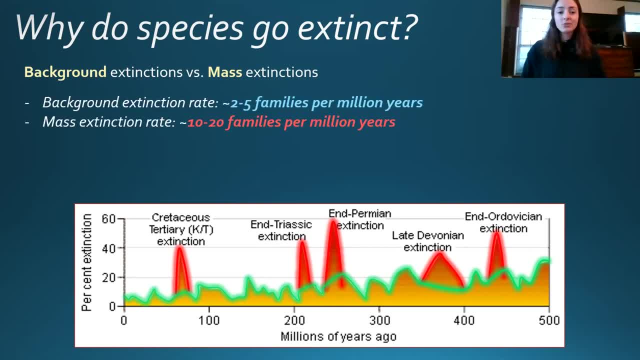 This green line is showing the background extinctions. This background extinction rate is about two to five families per million years, rather than mass extinction rates, which are about 10 to 20 families per million years. So the question is: are these huge peaks showing these? 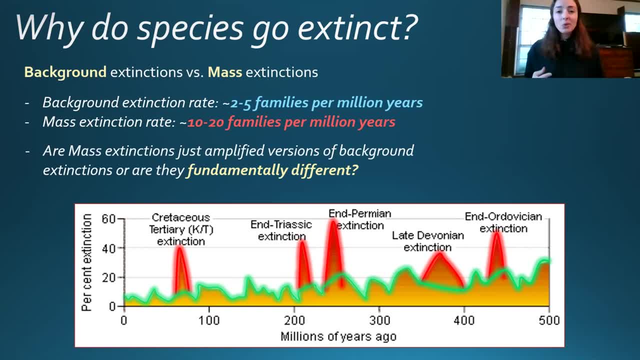 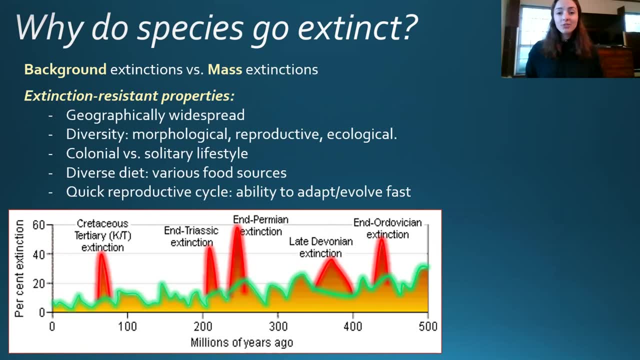 mass extinctions just amplified versions of background extinction, Or are they fundamentally different? What causes them, And is it different than what causes background extinction? In order to figure this out, some scientists decided to start looking at extinction-resistant properties. These include characteristics of groups of organisms or species, genera, families. 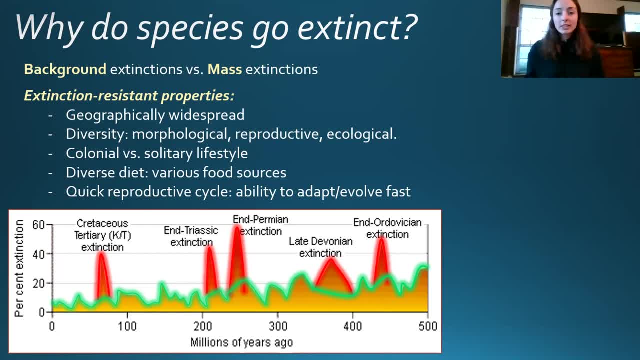 etc. that are geographically widespread. So if they're widespread, a catastrophe that happens locally may not totally wipe them out. Additionally, morphological, reproductive and ecological diversity. If you have morphological diversity you can adapt easier to different environmental. 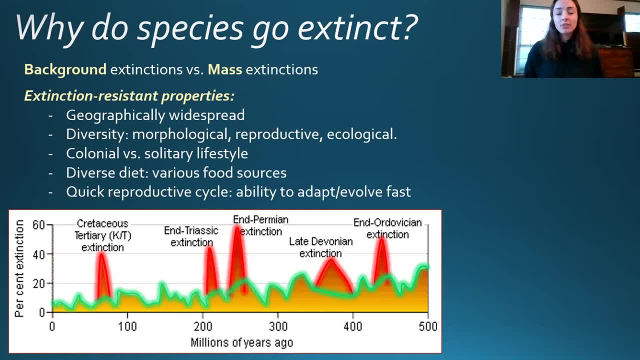 changes and different competition changes, etc. Reproductive diversity, like being bisexual, being able to release both eggs and sperm, and being able to be asexual in certain periods of time, depending on your environmental conditions and the ecological conditions that you're in, And so those things will help you survive in. 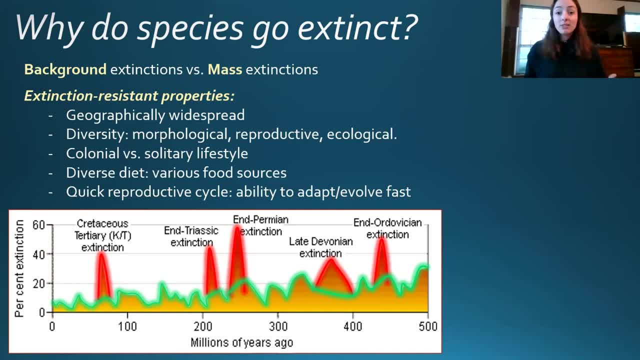 certain situations. Additionally, ecological diversity: being able to live successfully in different ecosystems, Colonial versus solitary lifestyles. Coloniality can be a very helpful evolutionary trait in order to survive in different situations that may break off a huge part of your animal structure, but then you can just regrow it by growing new individuals into your colony. 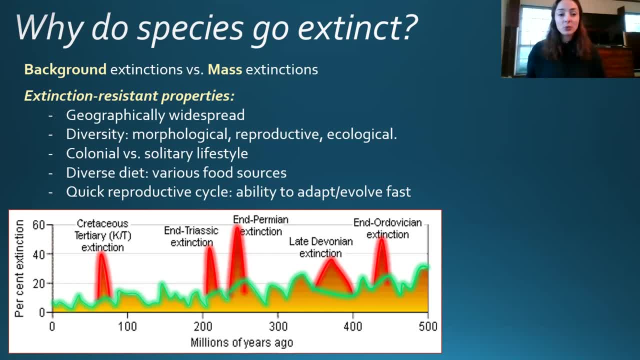 additionally, a diverse diet can help you adapt in different situations. Various food sources can help you not run out of food sources and still live in certain environmental catastrophes or competition situations that you may get into. And, lastly, a quick reproductive cycle and therefore, 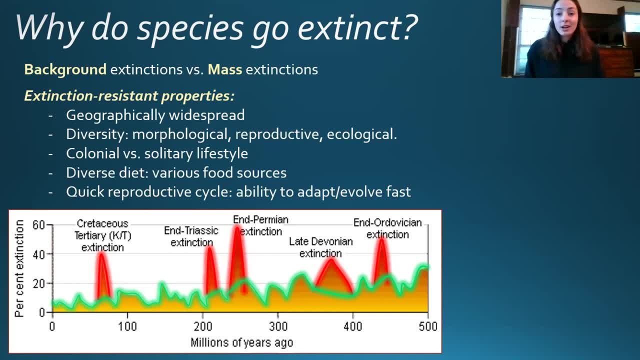 the ability to evolve or adapt quickly, Because if you take forever to actually go and have babies and raise them etc- kind of like humans do, it kind of takes a long time for you to actually evolve, Whereas if you're like a fruit fly or a mosquito, you're going to have millions of. 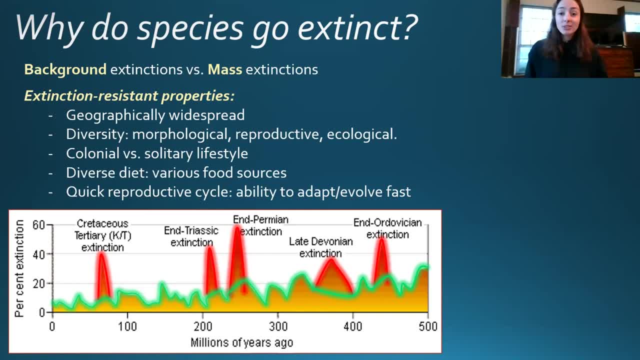 generations way quicker than humans could And therefore evolution can occur a lot faster And therefore if your environment's changing, then you changing and adapting along with it will be beneficial to your survival. So these properties are really important for background extinctions. 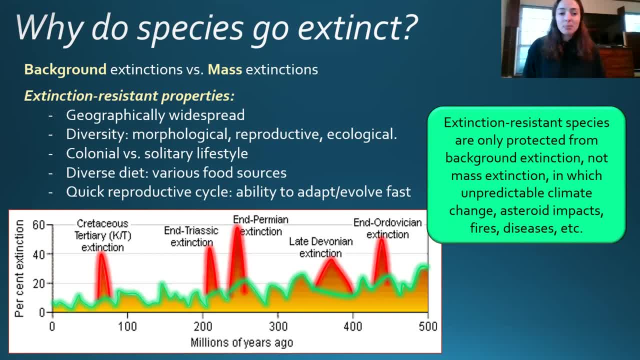 because the general causes of background extinctions are these typical competition and environmental situations that you might get into locally, but not globally. However, mass extinctions are more likely caused by unpredictable climate change after extinction, And so if you're in a global space or in a new day or age, it's not just that there's a global climate change, it's 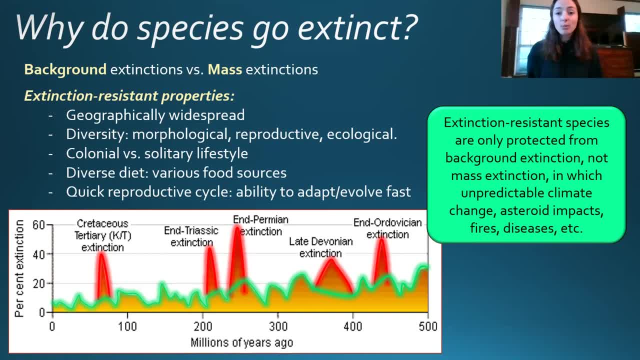 not just that there's a global climate change. it's that there's a global climate change. It's either a global catastrophe or it's unpredictable. It's an asteroid, it's a fire. it's something that the species can't really protect itself from, no matter how advanced it is, no matter how widespread. 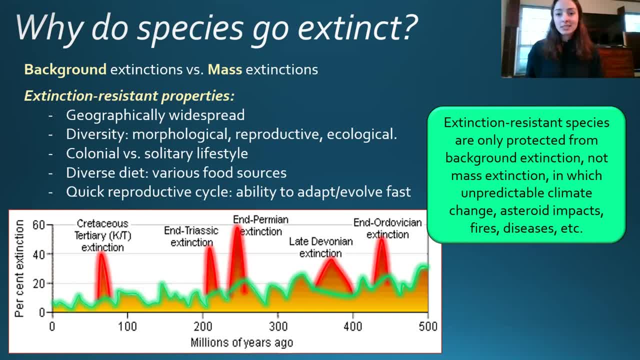 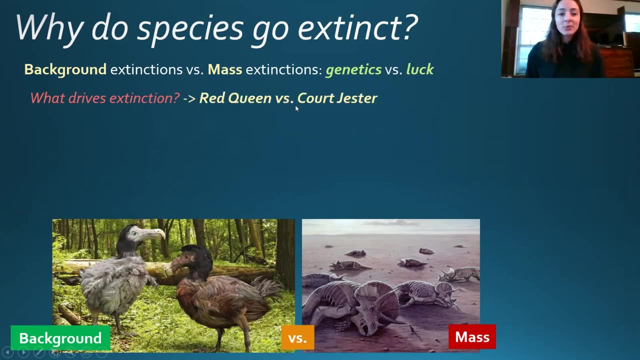 it is, no matter how diverse it is, It can't avoid mass extinctions, And so the general consensus here is that background extinctions happen to species with bad genes, and mass extinctions happen to species with bad luck. so now the question is: what drives extinction? so now, here we have to talk about the red queen. 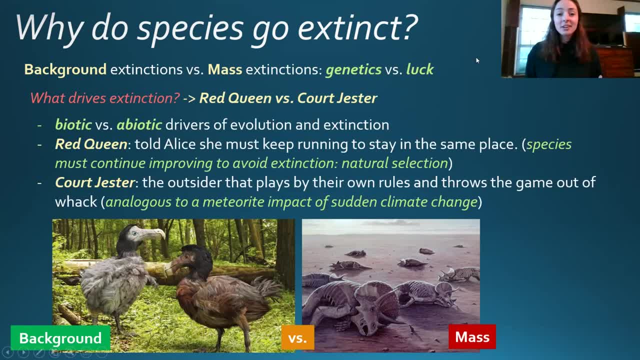 and court jester. what do these mean? basically, this is talking about biological versus abiotic drivers of evolution and extinction. the red queen refers to when the red queen told alice she needs to keep running to stay in the same place in alice in wonderland, which in this scenario, refers to. 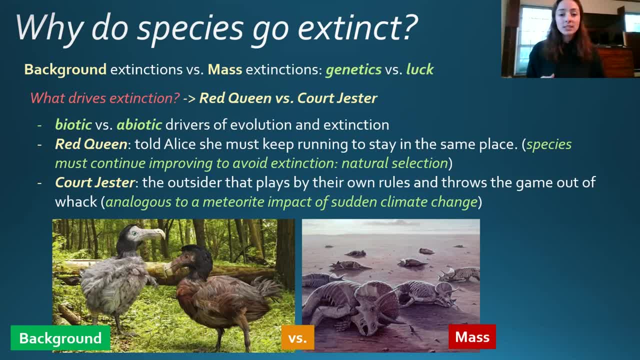 species needing to continue to improve to avoid extinction, which we talk about as the concept of natural selection. in the evolution and phylogeny video, however, the court jester refers to that outsider that plays by their own rules and throws the game out of whack, analogous to a meteorite. 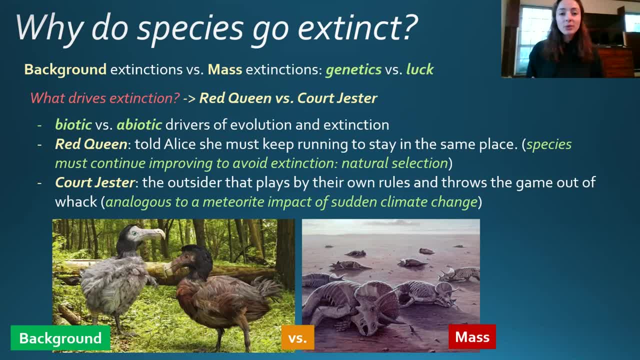 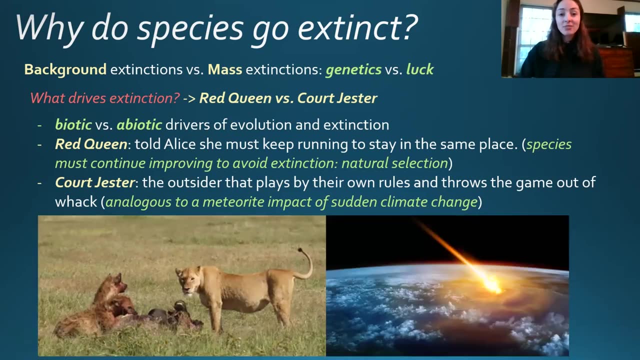 impact or sudden climate change, etc. and so the red queen versus court jester is similar to the scenario we were just discussing between background and mass extinctions. however, it's really controversial still in the study of extinctions which driver dominates- biological competition or abiotic environmental changes? however, 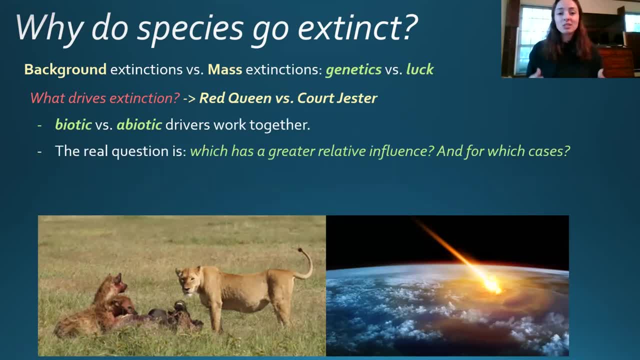 these are really intertwined factors. abiotic and biotic sources work together to drive evolution, by driving extinctions and creating new niches for new species to evolve, etc. and so the real question is: which has a greater influence, rather than which one is the driver? and another question: 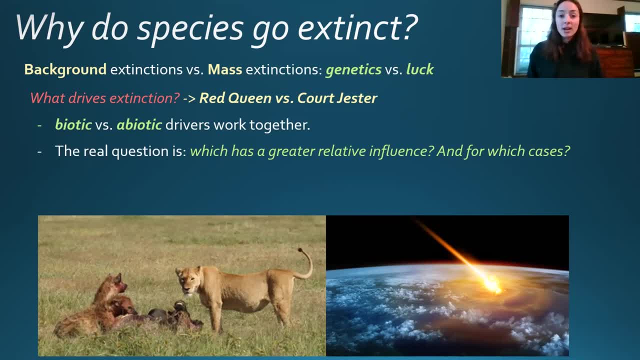 is for which cases do biotic causes drive extinctions and for which cases do abiotic causes drive extinction? like we mentioned earlier, there's a leaning toward the red queen driving background extinction and the abiotic court jester driving mass extinctions. but again, this is still a really controversial field with a lot of thriving research fields right now. 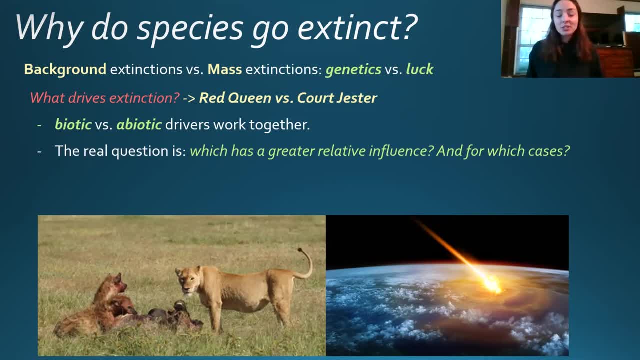 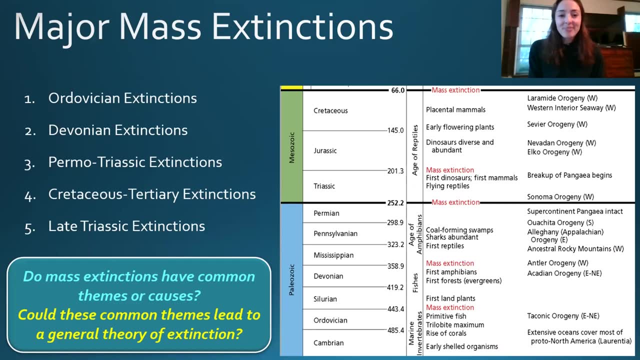 so if you're interested in researching extinction theory and understanding this more, i encourage you to look into it more on your own. so now getting to what i'm sure a lot of you are waiting for are the mass extinctions. the background extinctions just happen. these mass extinctions are really 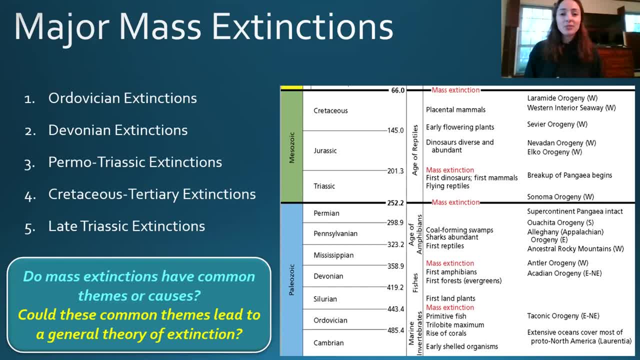 where it's all at. the mass extinctions include, like we mentioned earlier, the ordovician, the devonian, the perma-triassic, the cretaceous tertiary and the late triassic extinctions. this was supposed to be in order but pretend like number five, the late triassic. 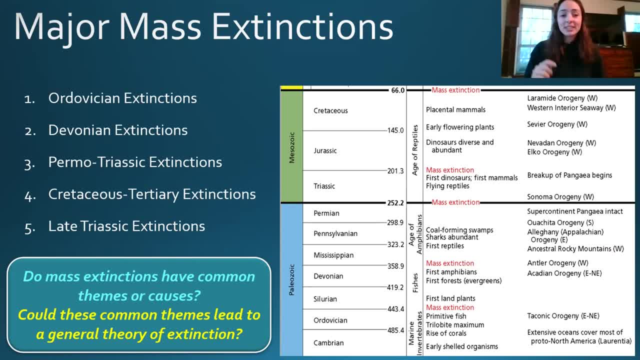 extinctions is supposed to be number four and pretend cretaceous tertiary is number five. sorry about that. so anyway we can see in the figure to the right where we have this time scale from the paleozoic to the mesozoic. we have the first mass extinction in the late ordovician, going into the 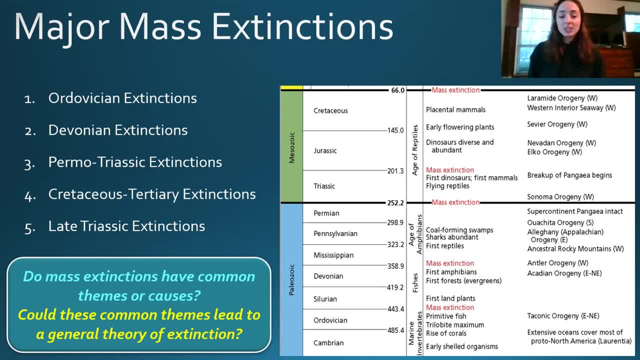 silurian, and then we have the devonian to mississippian extinction, and then the perma-triassic, the late triassic and the cretaceous tertiary extinction. all of these extinction events, you might notice, tend to happen at boundaries in the geologic time scale. why is this? it's not a coincidence. it's because 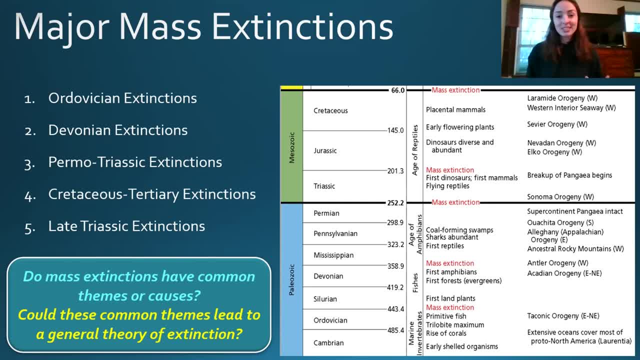 we knew about the fossil record before we actually put together the geologic time scale. we actually segmented the time scale based on the fossil record. and so when we look at the big perma-triassic extinction and cretaceous tertiary extinction, we see in the fossil record, in the rock record. 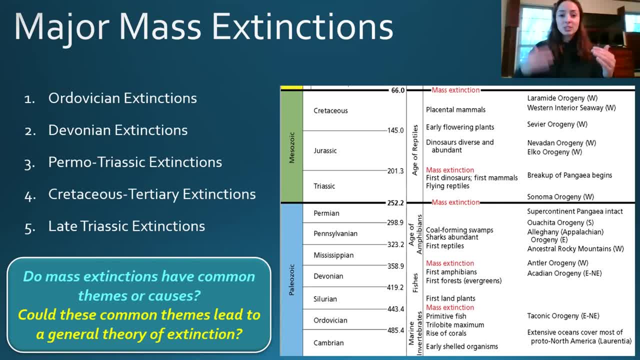 these huge differences in fossil content from the cretaceous to the tertiary and the permian to the triassic and the perma-triassic to the late triassic and the perma-triassic to the late triassic. because of this, people put a huge boundary there and said: this is a boundary between eras and that's. 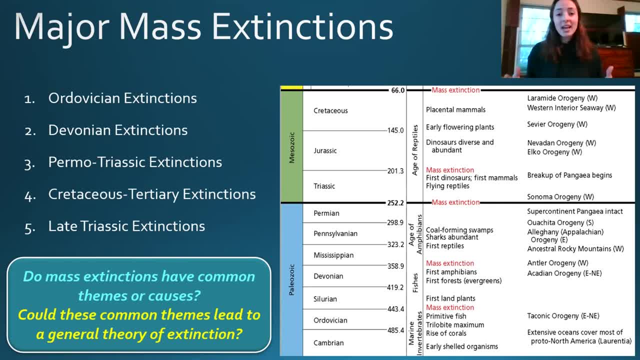 generally, how we made the geologic time scale and why all of these extinction events happen at these boundaries. so now the questions i want you to keep in mind as we move through these major mass extinction events and what caused them are: do mass extinction events have a common theme or cause and 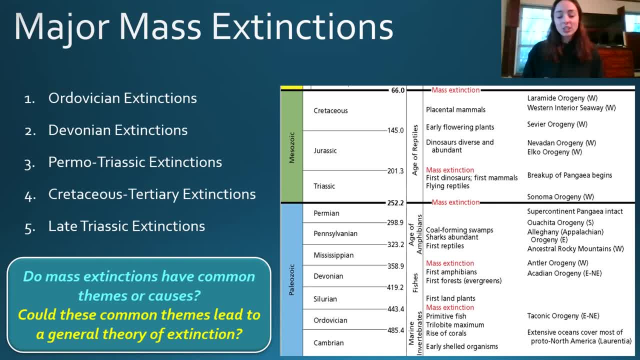 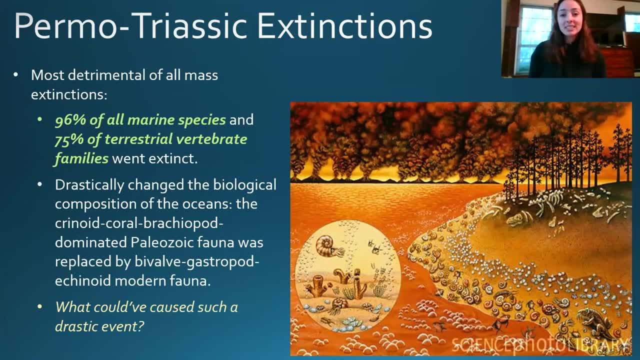 also, could these common themes lead to a general theory of extinction? first we'll talk about the perma-triassic extinctions. this was the most detrimental of all mass extinctions and because of this it's nicked the great dying fun right. so during this event, 96 of all marine species and 75 of all terrestrial 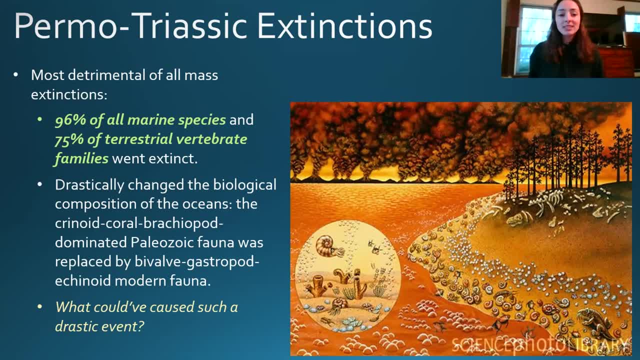 vertebrate families went extinct. during these extinctions, this drastically changed the biological composition of the oceans, converting the crinoid, coral, brachiopod- typical paleozoic faunas into bivalve gastropod, echinoid, modern fauna that dominate today. so what could have? 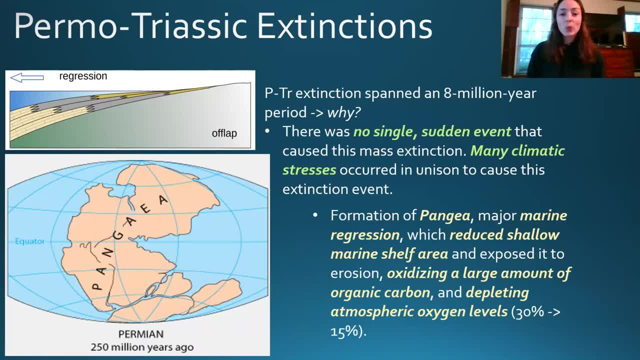 caused such a drastic event. well, it's not as simple as just one cause, and this event actually spanned an eight million year period, and so you might think the word event doesn't sound so applicable now. eight million years is a long time, so why did it span so long? 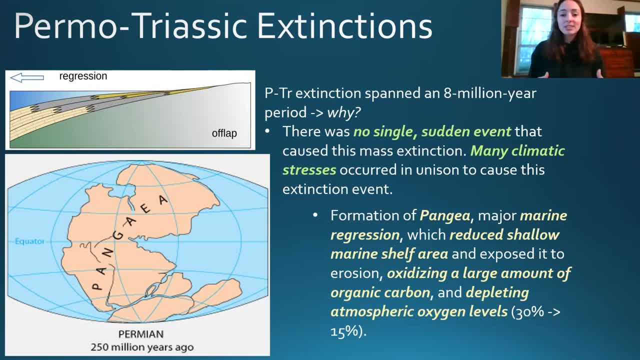 well, instead of one single event, there were many climatic stresses that occurred over these eight million years and came together to cause this major extinction event. these include major cause one which was major marine regression due to the formation of pangea, which caused reduced shallow marine shelf life and the extinction of the marine species. and the extinction of the marine species. 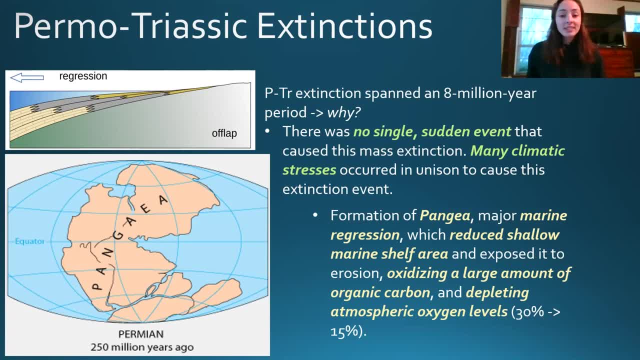 and also exposed it to erosion, oxidizing a large amount of organic carbon, releasing a lot of carbon dioxide into the atmosphere, as well as depleting the atmospheric oxygen levels, going from 30 to 15 percent, which is a lot of percentage to lose of oxygen. so that's one major cause of 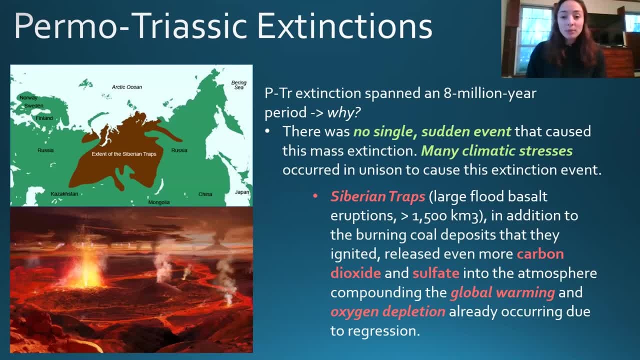 this extinction event. additionally, we had the siberian trap eruptions. these were large flood basalt eruptions which consist of a volume of over 1500 cubic kilometers, and they were, and in addition to erupting and releasing a lot of carbon dioxide and sulfate, just from the 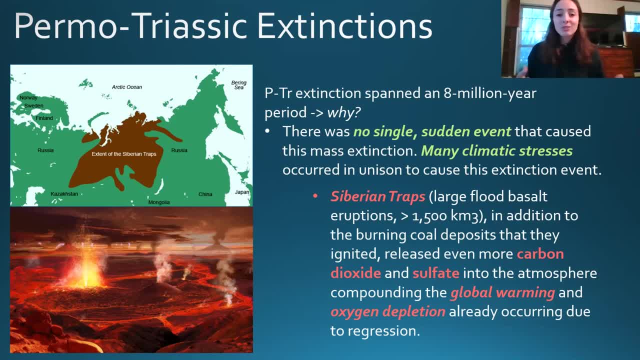 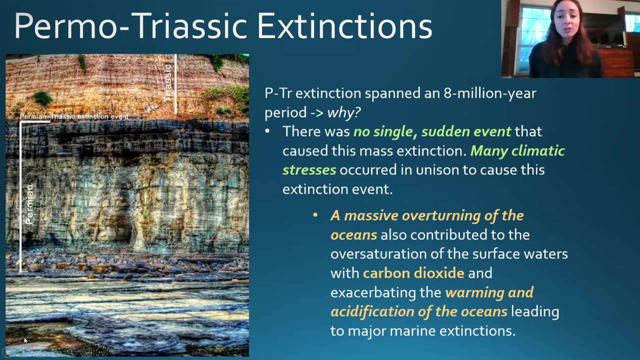 volcanic eruptions. they also ignited huge, extensive coal deposits, which burned even more carbon and released more carbon dioxide in the atmosphere, and this compounded the global warming and oxygen depletion of the atmosphere that was already caused by regression. additionally, a massive overturning of the oceans has also been seen in the rock record during this period, and this would 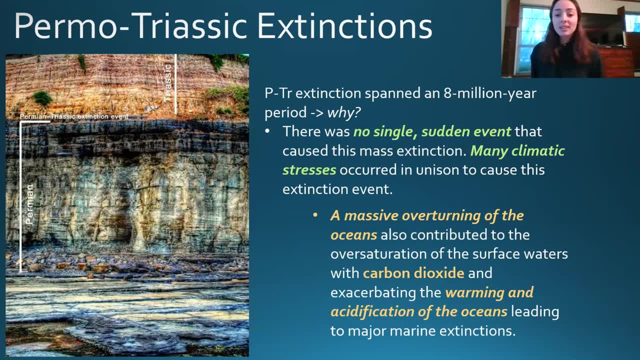 have contributed to the oversaturation of surface water through the ocean and this would have with carbon dioxide and also depleted the surface waters of oxygen, further depleting the atmosphere of oxygen and also exacerbating the global warming during the period and the ocean warming and the 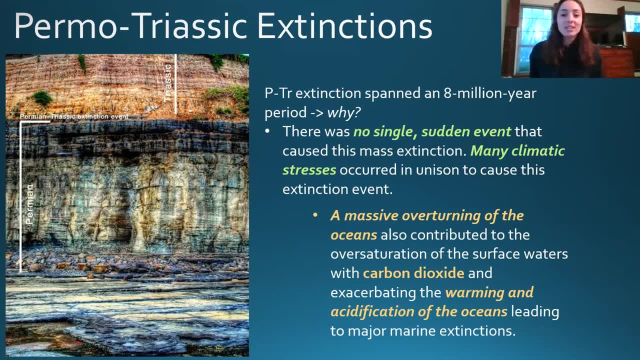 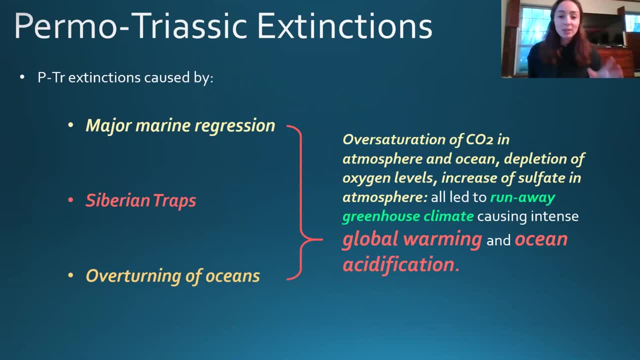 acidification of the ocean and leading to major marine extinctions, which is why we saw 96 percent of marine species go extinct during this time. so the marine regression, siberian traps and overturning the ocean in summary, caused an oversaturation of co2 in the atmosphere and ocean. 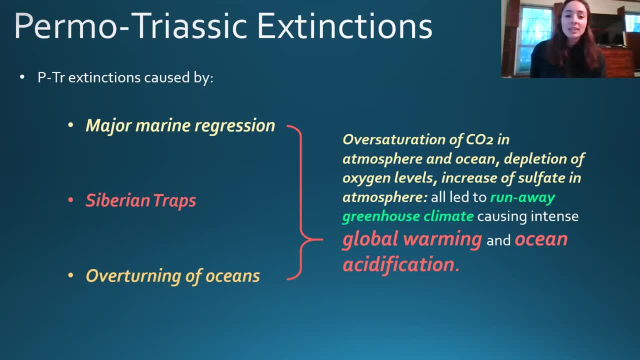 depleted oxygen levels and increased the amount of carbon dioxide that was released into the atmosphere, all leading to a runaway greenhouse effect, causing the intense global warming and ocean acidification that caused all these species to go extinct. the next mass extinction we'll talk about is the cretaceous tertiary extinction. this extinction event probably received the most. 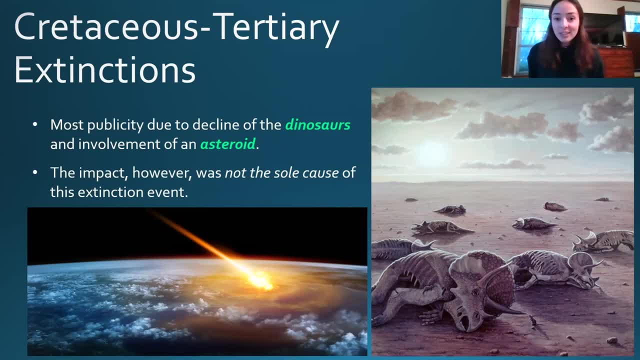 publicity because of the decline of dinosaurs. i don't say extinction of dinosaurs here, for a reason: they did decline and they were mostly wiped out. the birds are dinosaurs, so they're not extinct. and the other reason it receives publicity is the involvement of an asteroid. the impact, however, was 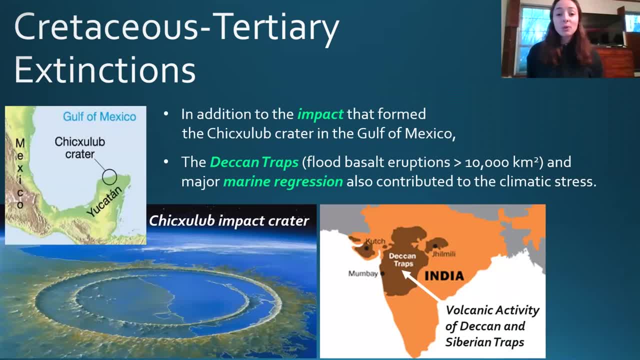 the only cause of the extinction, in addition to the impact that formed the chiksa loop crater in the gulf of mexico, shown in the images on the bottom left of the slide, the deacon traps, which are located in modern day india, shown in the figure to the bottom right, these flood basalt eruptions. 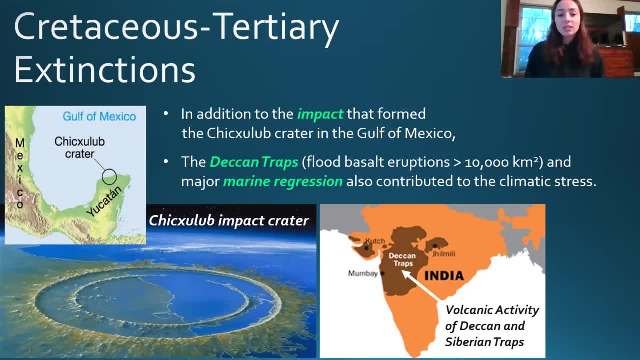 as well as major marine regression, again also contributed to the climatic stresses that caused this extinction event. the flood basalt eruptions themselves spanned an area over 10 000 square kilometers. the bottom label is wrong. i say deacon and siberian traps. it's supposed to just be deacon. 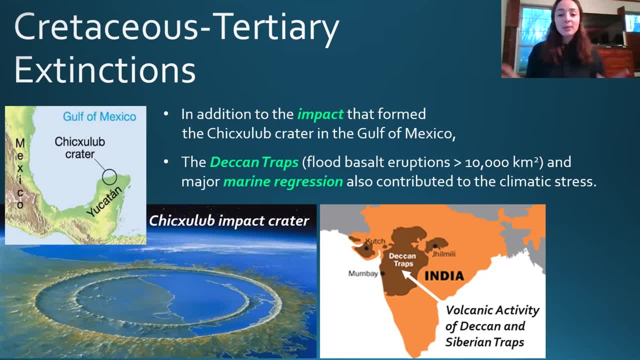 traps. we already talked about siberian. that was the perma-trassic extinction, but anyway, these deacon traps, like the siberian traps earlier in earth's history, caused a lot of co2 release, sulfate release, etc. marine regression caused reduction of shallow marine shelf area and the 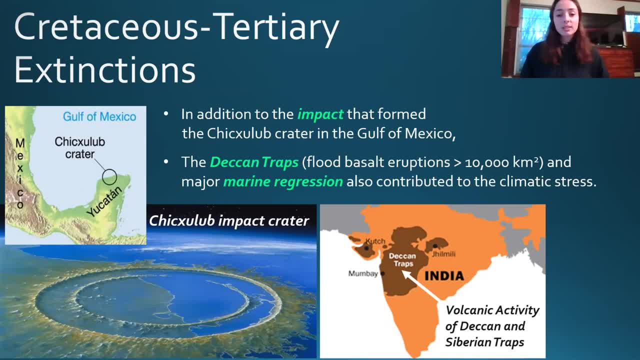 impact of the crater caused the blocking of sunlight, the endophotosynthesis, etc. and all of these factors, similar to the perma-trassic extinction, came together to ultimately cause the deacon and siberian traps to be deacon traps. the next extinction event we'll be talking about is the devonian extinction, which wiped out 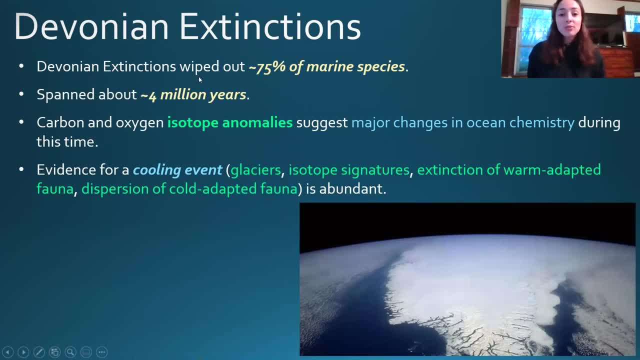 75 percent of marine species. this spanned about 4 million years and there's carbon and oxygen isotope evidence that suggests major changes in ocean chemistry during this time. the evidence actually suggests a cooling event, not a warming event, for this extinction, and this evidence includes glacial evidence, isotopic signatures, extinction of warm adapted fauna, but dispersion. 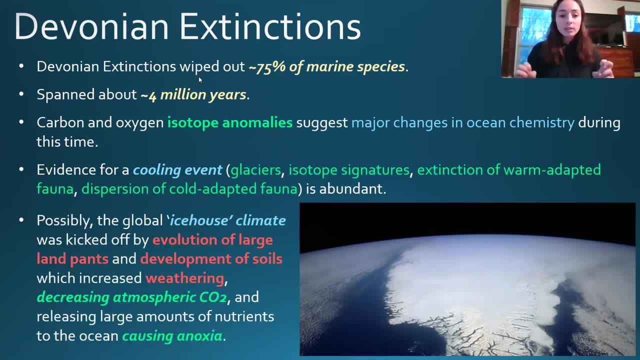 of cold adapted fauna toward the tropics, and this extinction event is a major extinction event, also known as the ice house. climate was possibly kicked off by the evolution of large land plants that caused the development of soils, which increased weathering, decreasing atmospheric co2 by both weathering and photosynthesis, and then releasing large amounts of nutrients to the oceans. 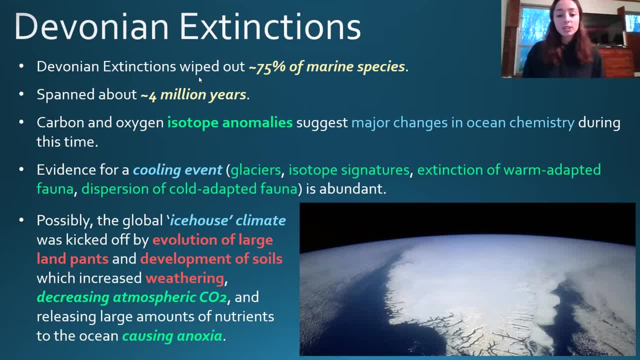 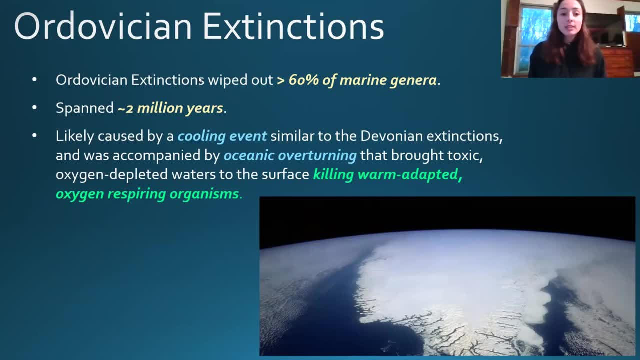 causing anoxia in the oceans or oxygen depleted conditions. likewise, the ordovician extinctions, which wiped out 60 percent of marine genera and spanned 2 million years, was also likely caused by a cooling event and was accompanied by a few more of the most event-like and highly toxic 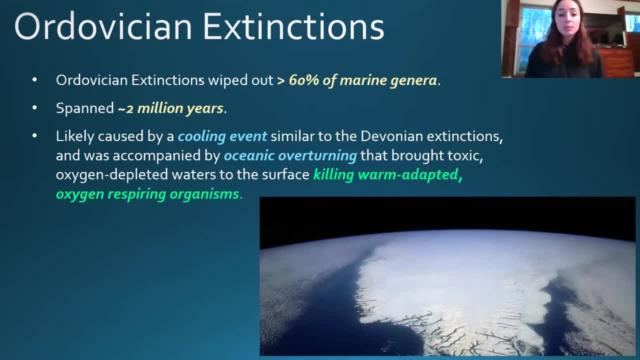 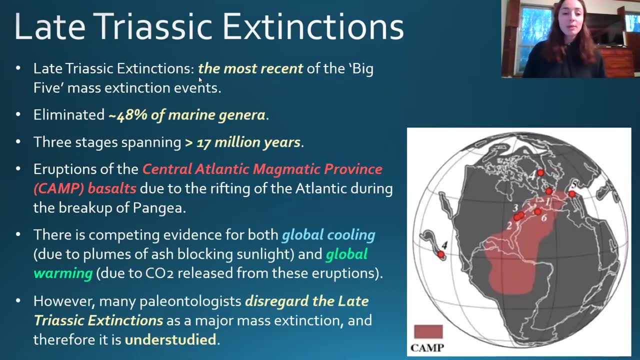 by oceanic overturning, which brought toxic, oxygen-depleted waters to the surface, killing warm-adapted and oxygen-respiring organisms. The last major extinction event we'll talk about is the Late Triassic Extinctions, which is the most recent of the Big Five mass extinctions. It is 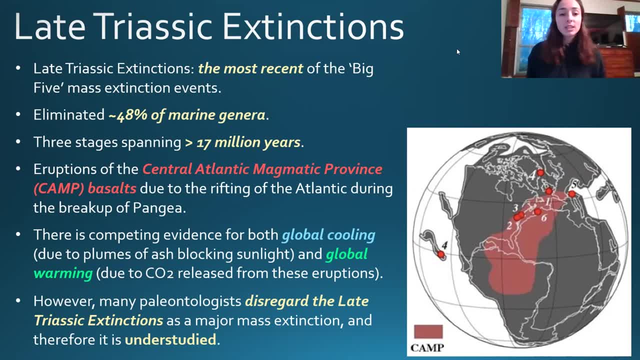 estimated that it eliminated about 48% of marine genera and spanned over 17 million years, with three stages. It is thought that the Central Atlantic Magmatic Province, or Camp Basalts, began erupting during this period due to the rifting of the Atlantic during the breakup of. 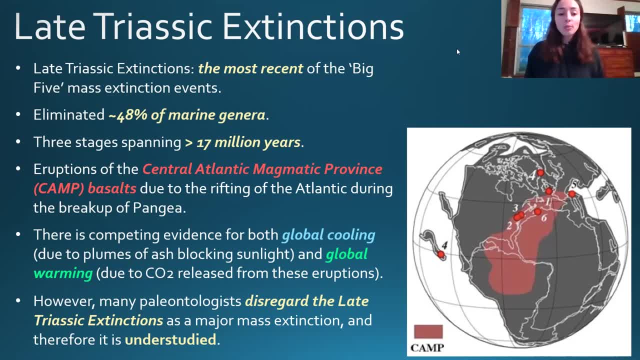 Pangaea. There is actually competing evidence, though, for both global cooling due to plumes of ash from these volcanic eruptions that blocked sunlight, and global warming due to CO2 release from these eruptions during this time, So this is actually a more controversial extinction event. 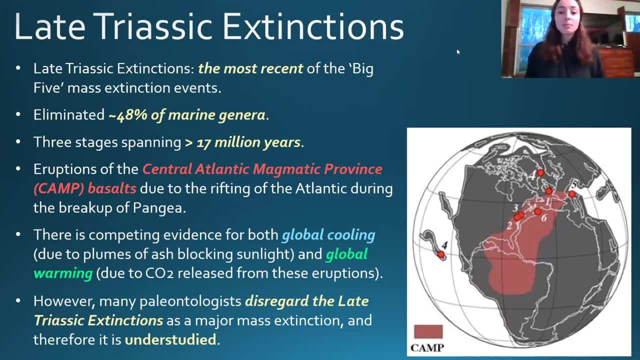 and it's still uncertain what actually caused it. Some people think that it was actually both climate changes- cooling and warming- that happened right after one another to cause rapid climate change, which species just couldn't keep up with. However, many paleontologists disregard these Late Triassic. 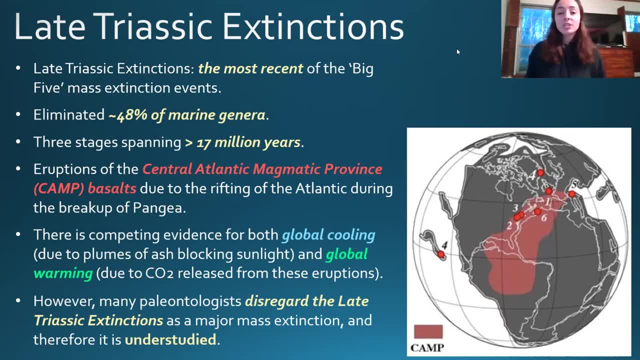 Extinctions as a major mass extinction and instead they think it's just a statistical anomaly that the extinction rate spikes in the plots of this data due to how statistically these extinctions are clumped and therefore it is understudied. So now that we've talked about 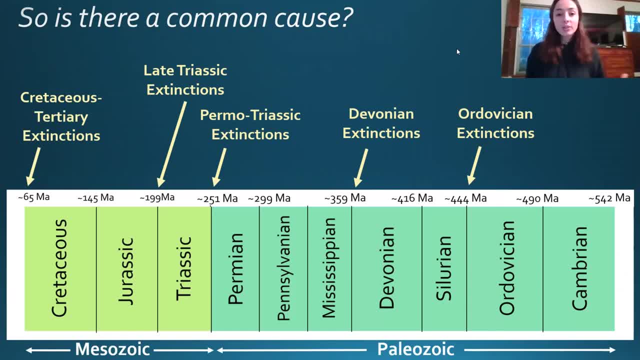 the Big Five mass extinctions, and here we see when they all occurred, on a timeline in order. we can ask the question now: is there a common theme or cause to all of these mass extinctions? I mean yes, in the way that we saw similar climatic stresses occurring in each. 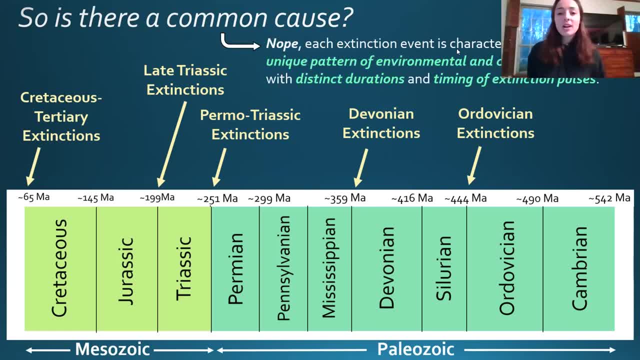 situation, However, no, not in the big picture and not that will actually lead to a theory of extinction. Each extinction event is characterized by a very unique pattern of environmental climatic fluctuations that were really random in their order and their placement throughout the geologic. 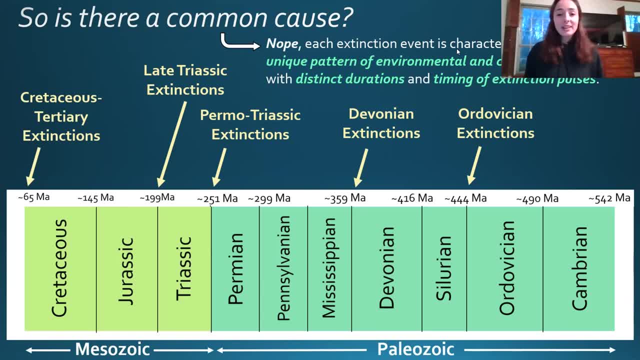 timescale, showing that it's more just serendipity than anything. And so, because of the unique pattern of environmental and climatic fluctuations, with unique durations and timing of extinction pulses in each one of these events, we can't make any statistical. 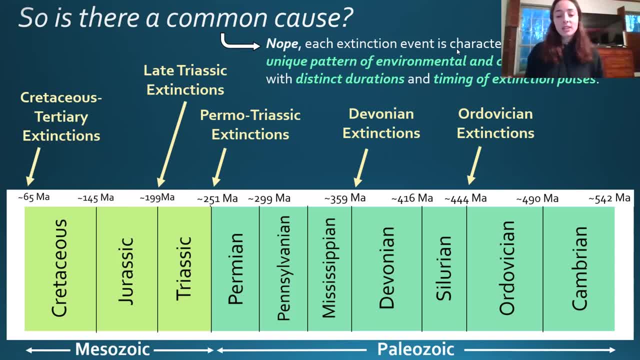 inferences or theories of extinction based off this. So even though we can take from it a little bit like CO2 excess in the atmosphere is a bad thing, we can't actually make an entire theory of extinction based off any common themes in these extinction events. So that's all I have for you. 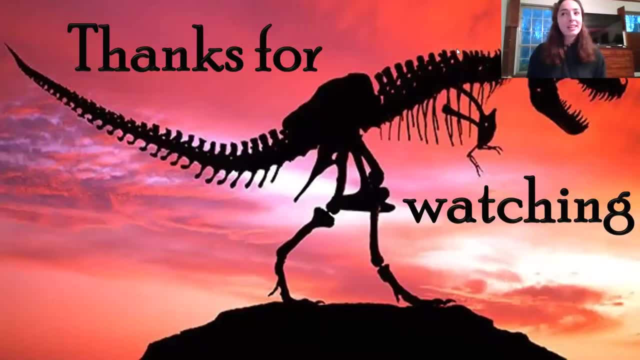 guys, today I hope you enjoyed learning a little bit about extinction and just kind of the causes of extinction And if you want me to make a more detailed video about the causes of extinction, about the sixth mass extinction that is currently occurring or any one of these mass extinctions. 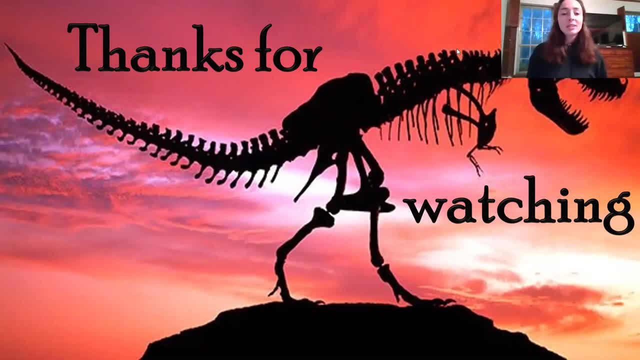 that I didn't focus too much on, then please let me know in the comments. And also keep in mind that as you're watching this, make sure you try and remember which periods the mass extinction has occurred in, because that will help you later down the road when you